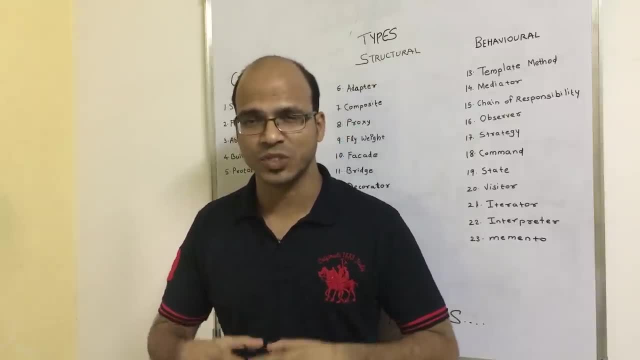 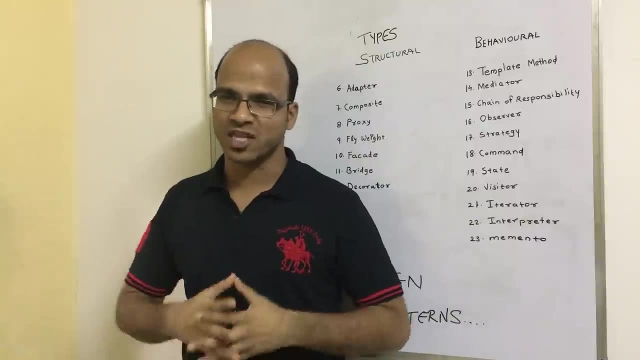 Welcome back aliens. this is Navin Reddy from Telescope Learnings, and today we'll discuss something about design patterns. Now you know when you, you can build your own software, right, of course, anyone can build a software and to to develop a software. what we should know is: 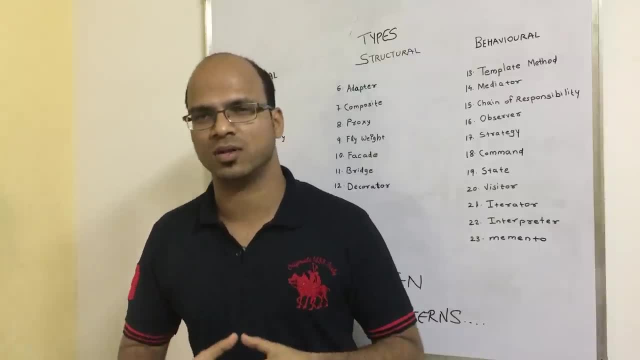 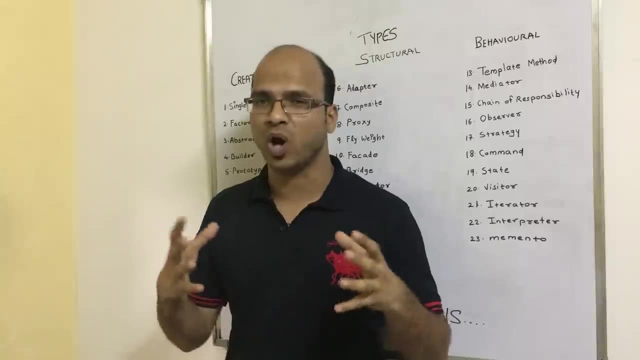 programming language right, and one of the best language to learn so that you can build a software is java, of course, right now, let's say you want to be a software developer, so what you will do? you will spend one week and then you will learn java, and the next week you will start making. 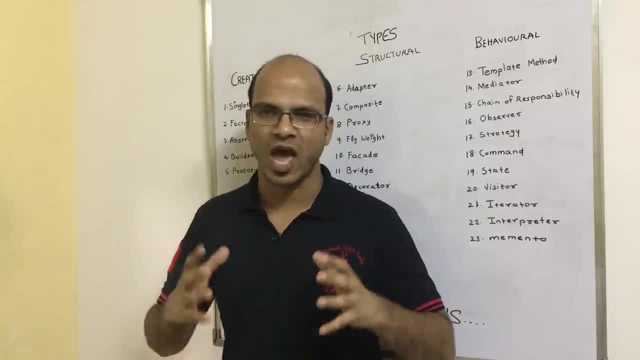 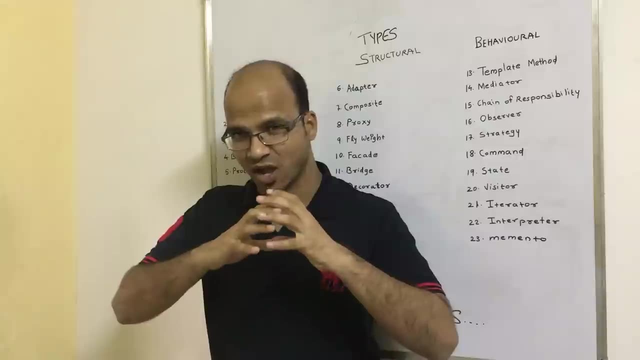 softwares awesome, right, but when you build a software, you have to face lots of problems. now, these problems: there are some problems out of this which are very common, problem which has which it which are faced by lots of software developers. so what if, if you have a common 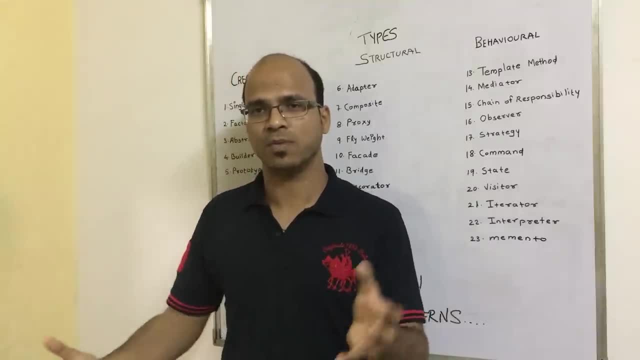 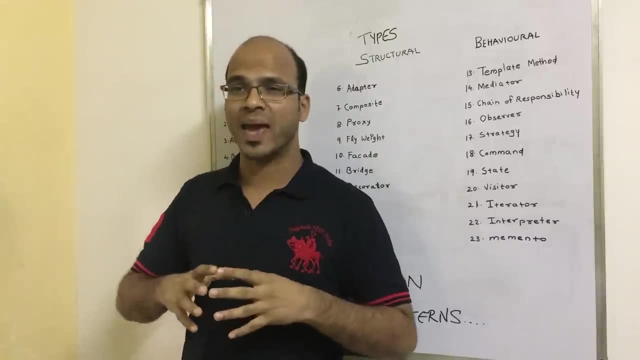 problem, can we just solve it and then anyone having the same problem can use that, can use that solution, of course. right, we can do that, provided that's not a domain problem, example, when you're working on a banking application, so that's a different domain when you're working with. 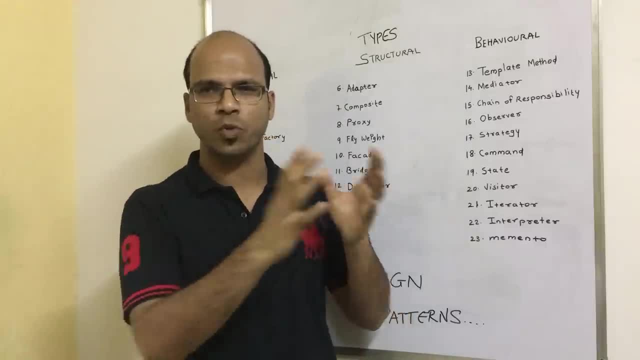 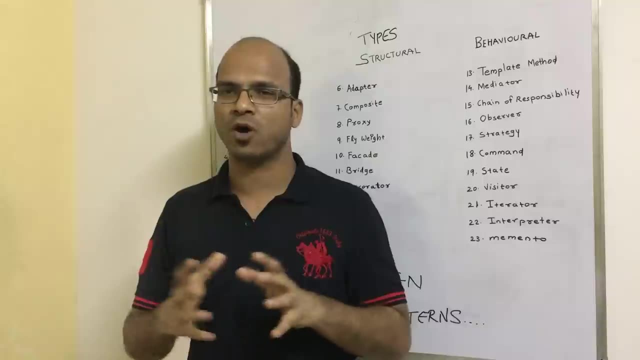 a, maybe a social networking app. that's a different domain. but if you talk about the conceptual- which is object orientated, conceptual problems, we can solve that with the help of some common solution, and now also throughout the industry we have some professionals. they provided something called as. 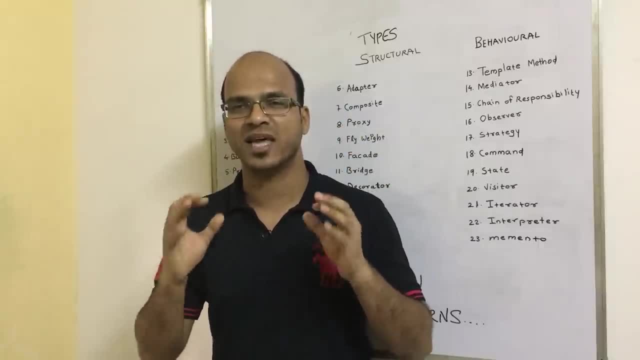 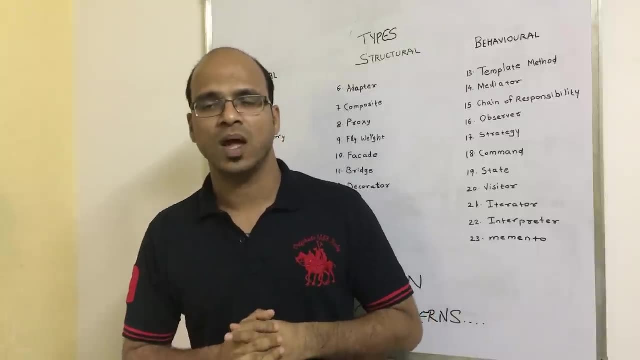 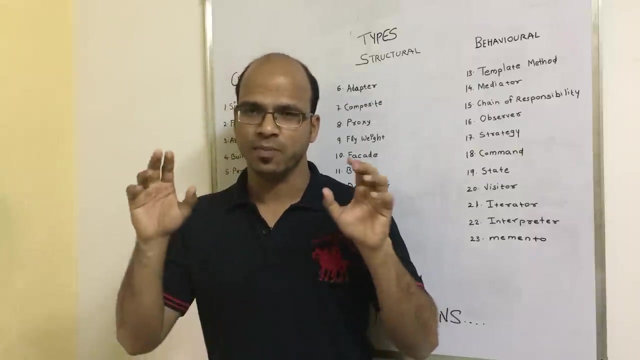 best practices and we call those best practices as design pattern. so it all started in 1994 around. so there was a book by four people and in which they have mentioned the principles of design pattern or principles of object oriented design patterns. so the main motto was just to so. 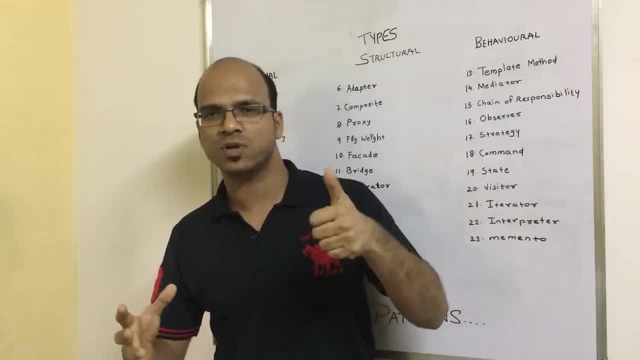 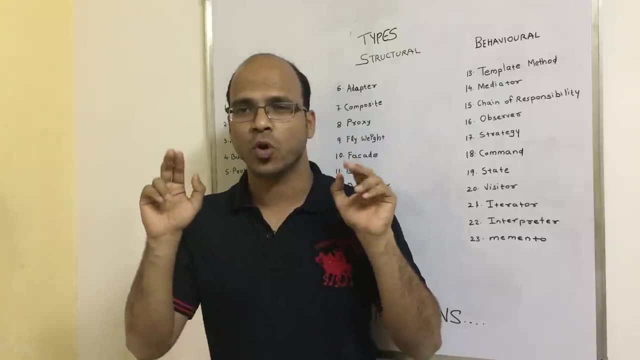 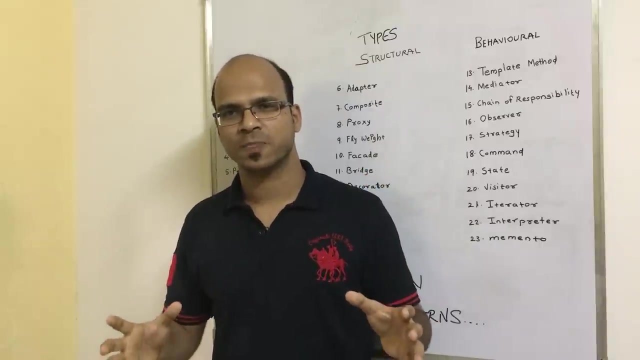 whenever you have a object oriented software, the first principle was: you should always prefer composition over inheritance, and the second principle was: whenever you code, code for interface, not for the implementation, and depend upon these two lines. they created the whole set of design patterns, and these four people were commonly known as gang of four. it's gone like. 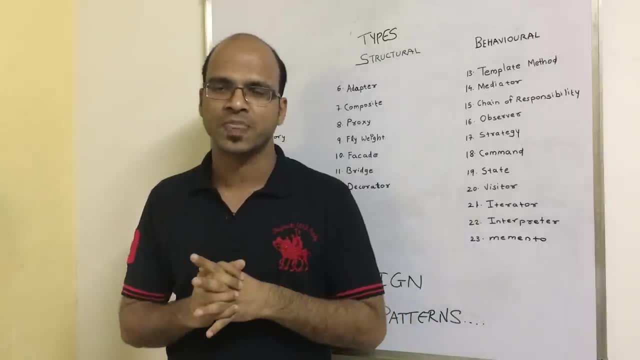 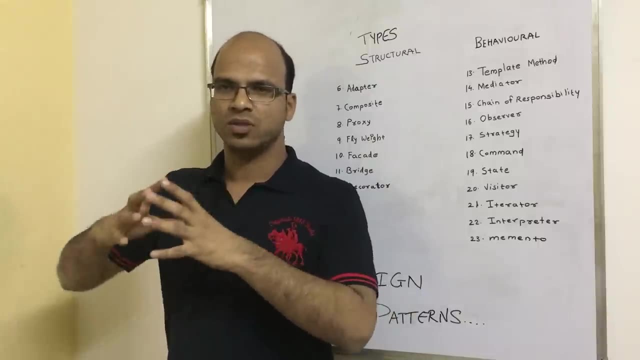 goons right. so we have gang of four people. so we have these four people and now, so they have defined some design patterns. so, and we have just classified those design patterns into three sections, so we have this struck: the creation design pattern, we have structural and then we have behavioral. so 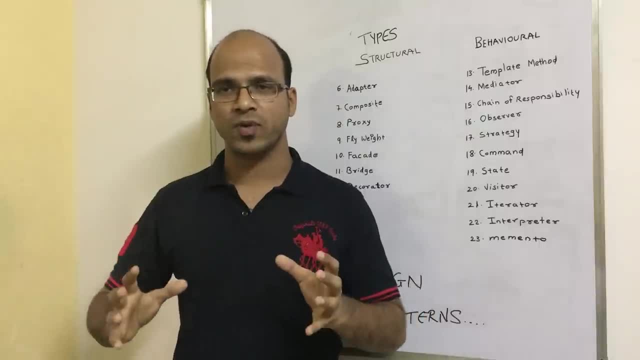 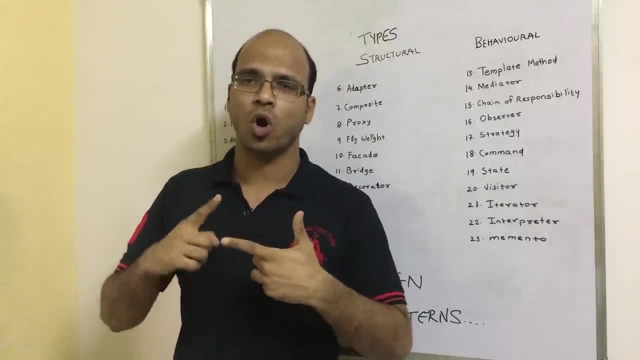 we have lots of design pattern right, so now, if you want to build a software using best practices, follow this design pattern. but there are two questions now. the first question is: should we know all design patterns? and the answer is yes, you should know all the design patterns. the 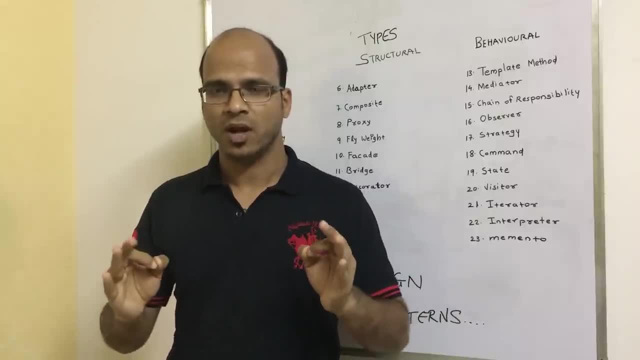 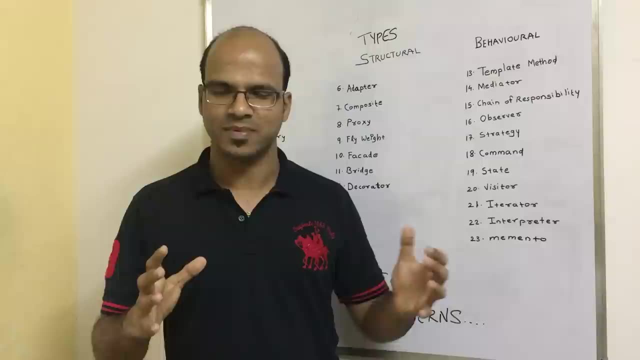 second question: should we implement all this design pattern? of course, right. so let's say you're. when you're building a next software now you will be using all design pattern, right. hold on, that's not the case. you should not use all design pattern in one software. it should depend upon your. 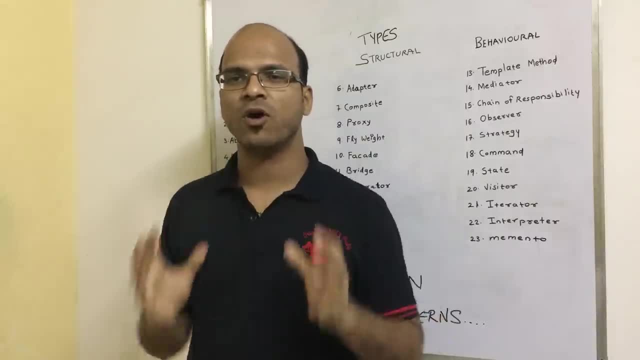 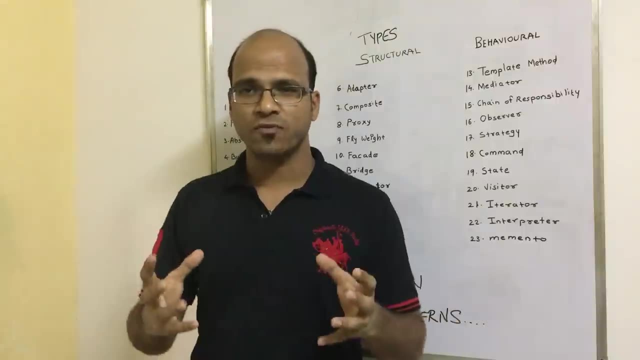 requirement. look at your requirement. if your requirement says we want to create an object, how to get an object, then we have to follow creation design pattern, right? let's say: i want to write a software in which you want to compose objects. so let's say you have an object inside that. 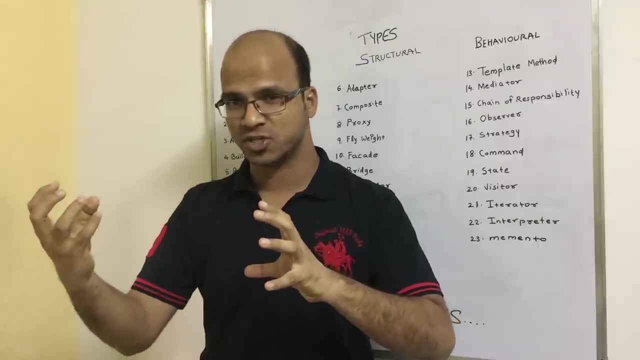 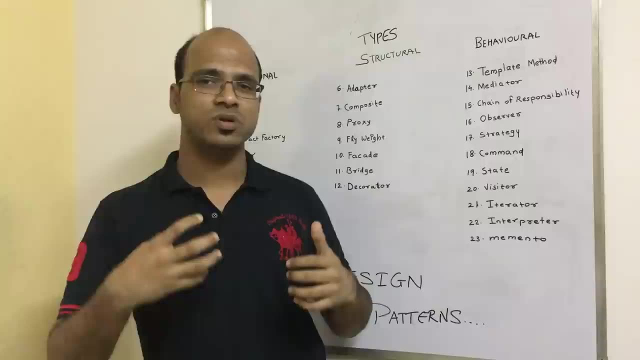 you want to include one more object, or if you have an object here which provides some features- you have object here which provides some features and this object wants to use this object- then we have to work with structural design patterns. the third one is: let's say you have 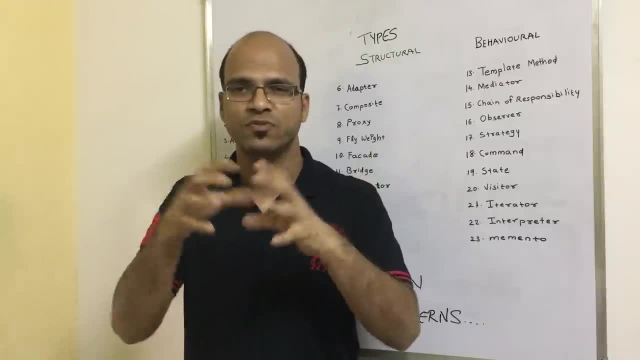 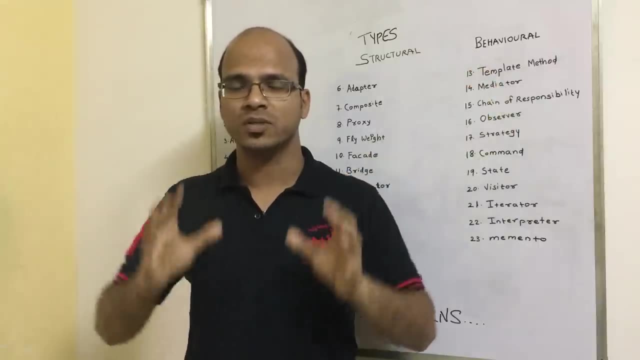 two objects. we don't want to compose them, but we want to make some communication between those two objects. at this point you have to use behavioral design pattern, right? so it's all depend upon your requirement. don't rush off, don't rush to use design patterns. think about your logic, or think: 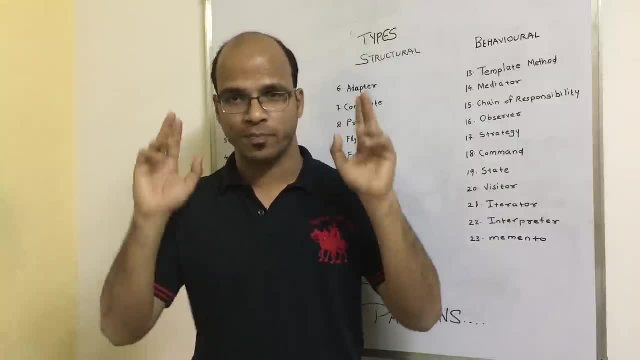 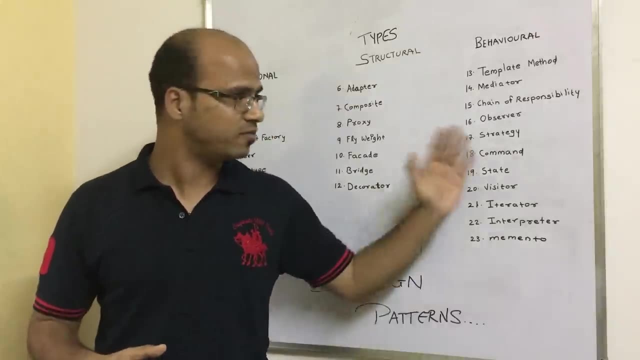 about your software problem. try to solve those problems with the help of best practices. which is design pattern here and you can use any of this. so approximately we have 13, 23 design patterns. we have some more, but this is basic design patterns you have here. okay, so let's start with the first. 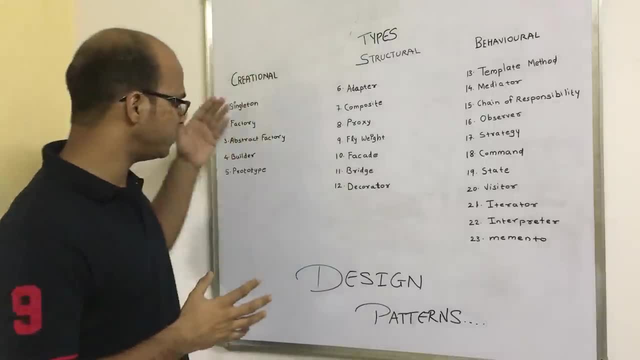 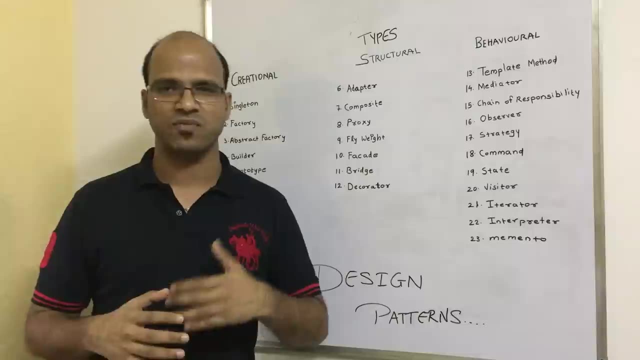 one. we have creation design pattern. so, in which you have six or five design patterns, one of the- my favorite- is factory pattern. so when you, if you're working with spring framework, if you're working with hibernate, you know about what is factory right. then we have singleton you can create. 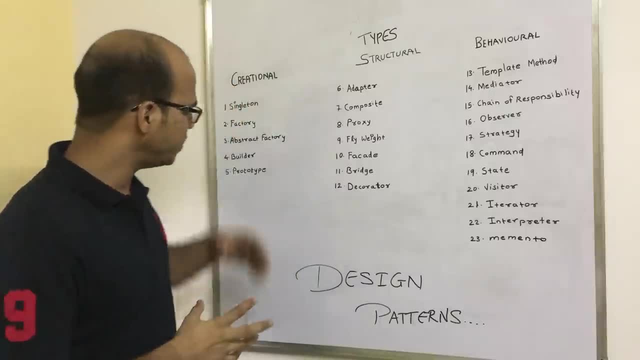 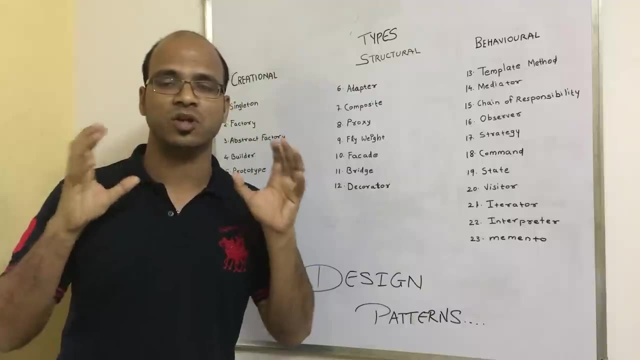 only one instance of a class. amazing right, don't know what use it now. so we have all the design pattern here for the creation, because here your concern is about creating the object. how to create an object, maybe using factory, maybe using singleton. so it's all about creation of the object. the next: